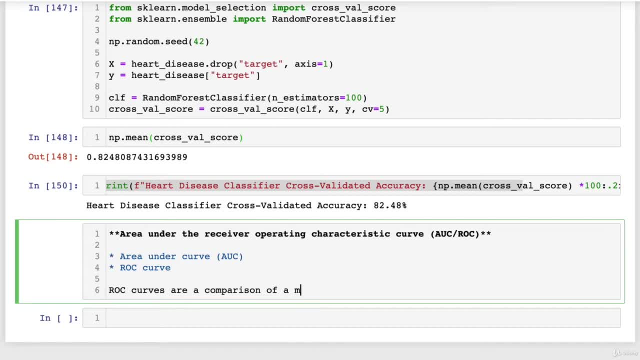 V1 comes out one and Y seems to be the less than or equal to true positive property. V1 comes out one and Y seems to be the less than or equal to true positive property of the modified systementeaching, which is a big. 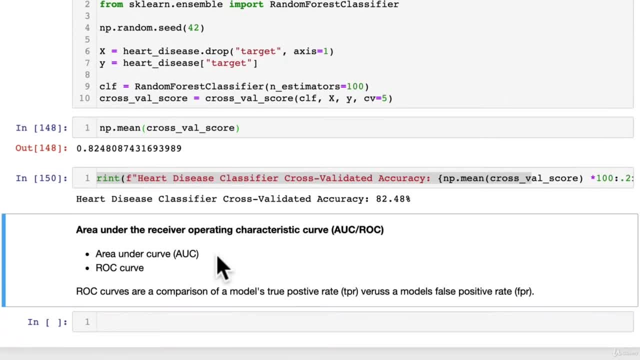 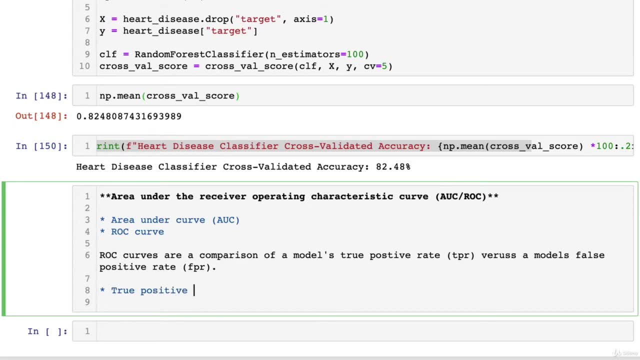 play-account TV position Y's. I mean upon doing all of this, all right, what happens? Well, you might have the longing to point out why positive and what is a false positive. well, let's have a look here. a true positive equals model. 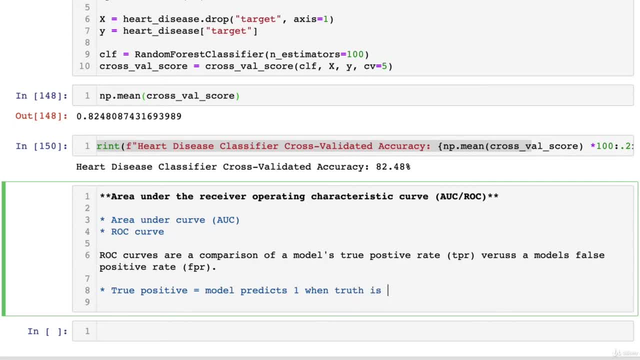 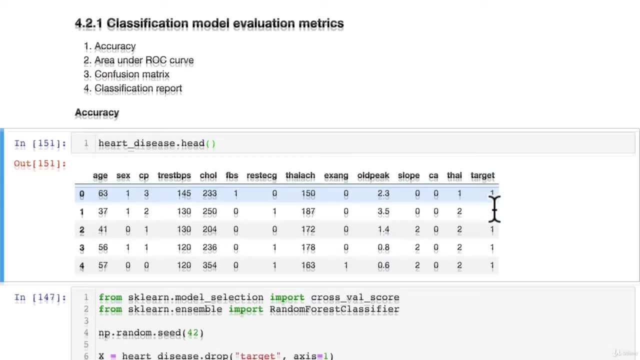 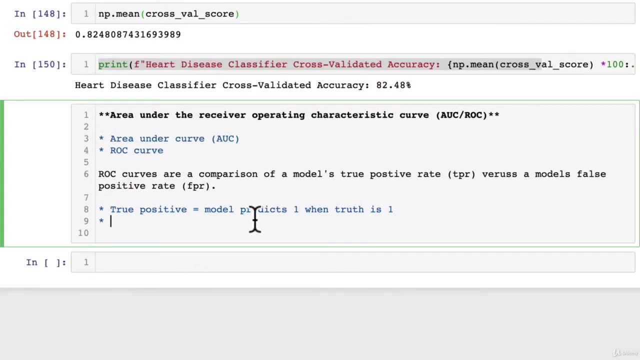 predicts one when truth is one. does that make sense? so in our case, if we have a look up here, if our targets are one or zero, a true positive is when our model predicts a one. the real label is a one. okay, yeah, that makes sense. so if we go here, a false positive is: model predicts one when truth. 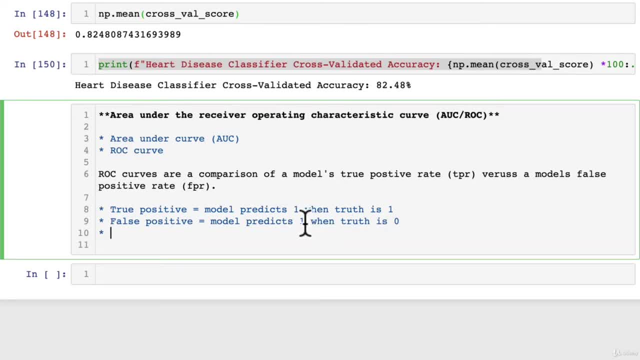 is zero. so why is it called false positive? well, it's because it's predicting one. so aka the positive class has heart disease, when the truth is actually zero. so it's giving us a false positive sense that that a person may have heart disease in in our particular case, for our heart disease, 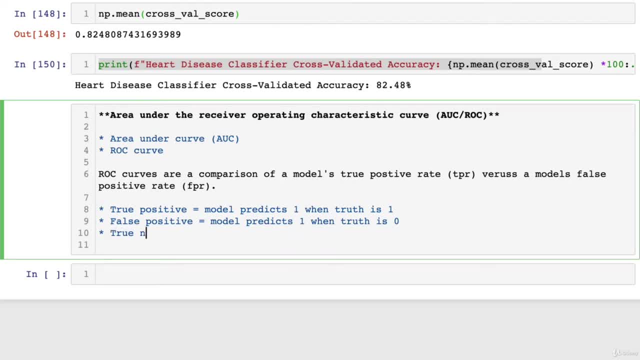 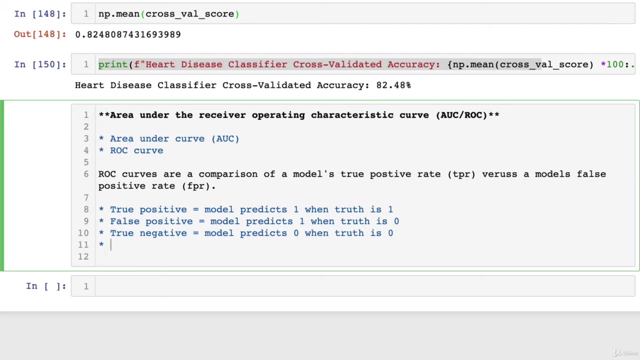 classification problem. and then, if we go here, a true negative equals model predicts zero when truth is zero. so that makes sense. so that's predicting. the model is getting the right prediction there. it's predicting someone doesn't have heart disease when they actually don't. that's great. and then a false negative equals model predicts: 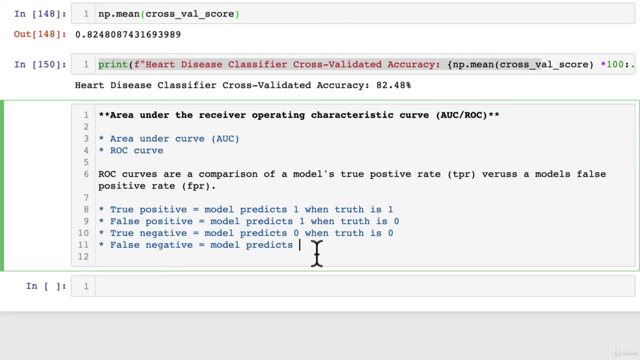 what do you think? this one will be false negative. we look at false positive. a false negative is when model predicts 0 when truth is 1.. So that's because it's predicting not heart disease when it actually is heart disease. So now we know these, We can see that a rock curve. 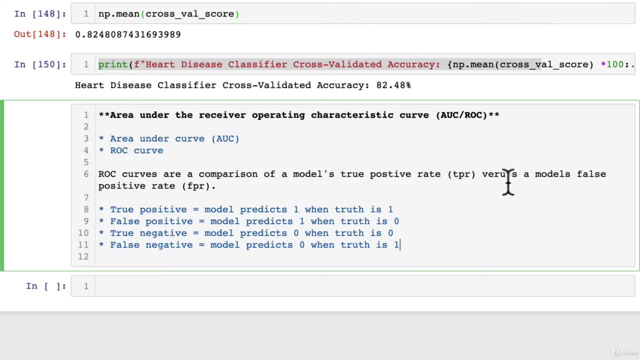 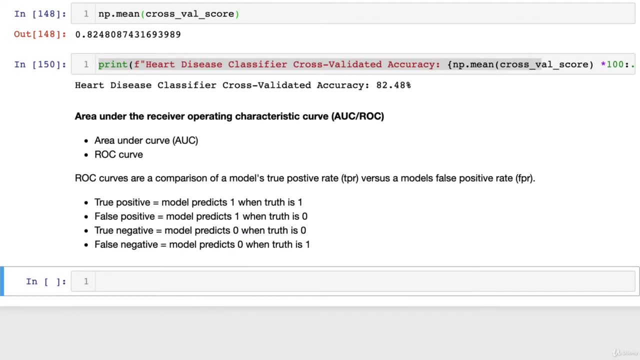 is a comparison of a model's true positive rate, TPR, versus typos everywhere here, Daniel, come on- versus a model's false positive rate or FPR. So now we know this, Let's see it in action. So we can do this using scikit-learn's. 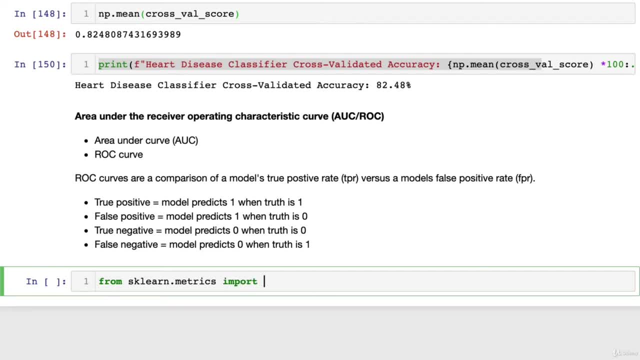 metrics library. We're going to import ROC curve, So see how I was saying rock curve, ROC curve. and then we're going to make predictions with probabilities. And how can we make predictions with probabilities? We saw this in making predictions. We can do that with yprobs. 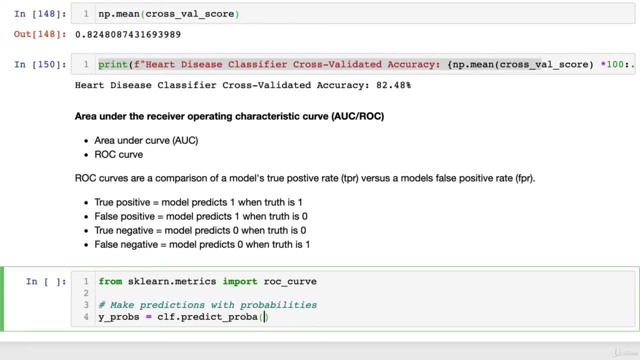 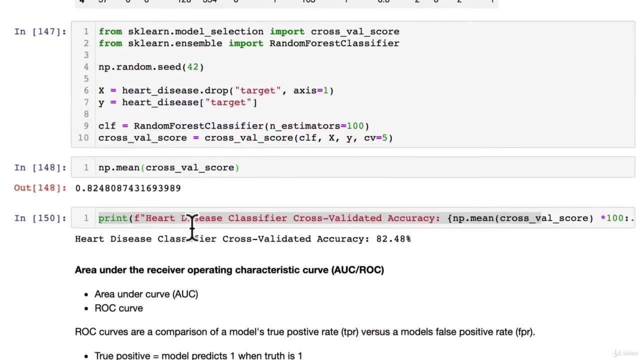 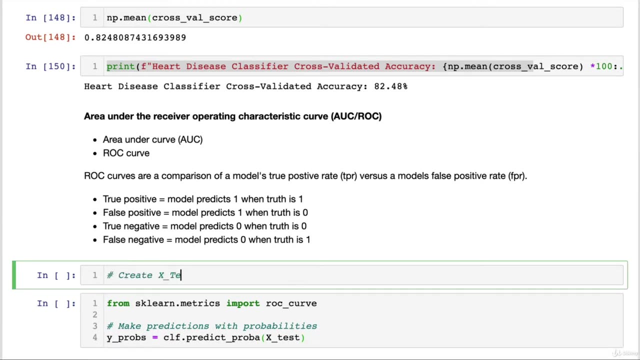 equals clfpredictprober for probability. We're going to make some predictions on the xtestdata Now I just want to make sure maybe we do that when we create xtest, just to make sure it's the right xtestdata, xtest, etc. So we want to go. 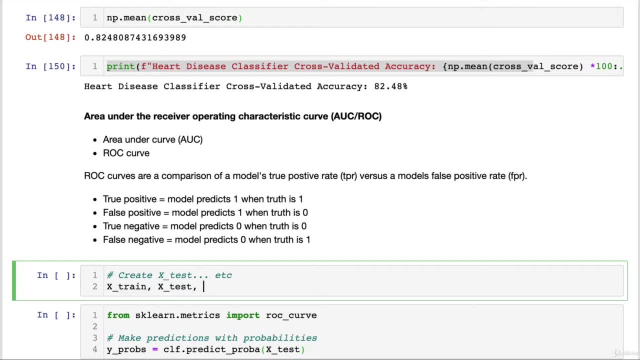 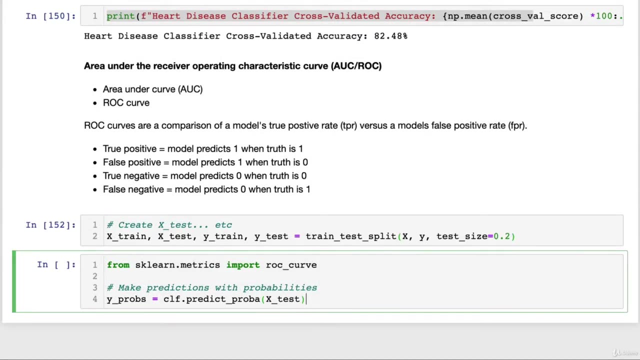 here: xtrain, xtest, ytrain, ytest equals train test, split, xy, Test size equals 0.. 0.2.. Wonderful, And so now we can do that there, Because a ROC curve is a comparison of a model's true positive rate versus a model's false positive rate. 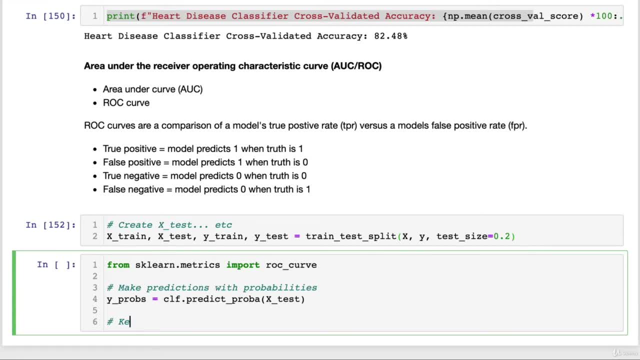 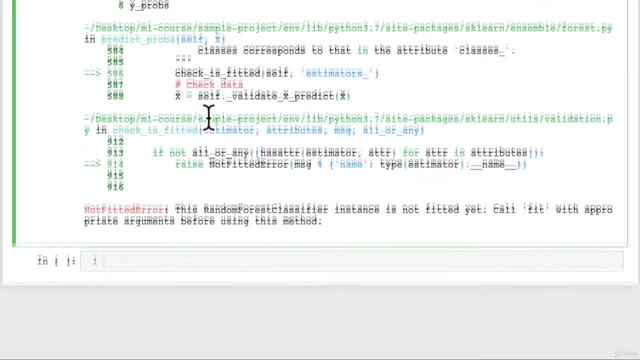 we want to only keep the positive classes. So actually, let's see what yprobs looks like. yprobs- why hasn't this worked? What do we got here? This random for is classified as not fitted, yet Call fit. Ah, that would make sense. So we want. 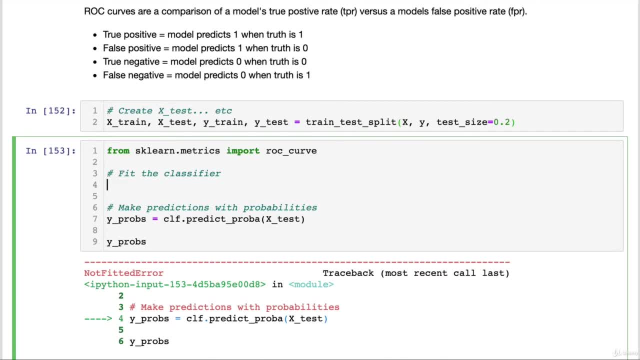 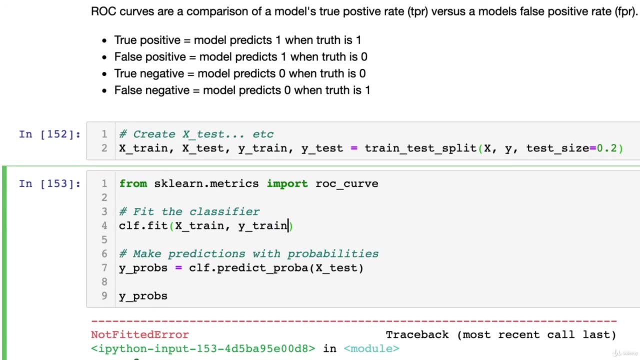 to fit the classifier. Of course you can't make predictions without fitting them, without the model learning any patterns. So we're going to fit it here. then we'll make some predictions and we'll have a look at this. Maybe only the first 10, so we're not taking up heaps of space. 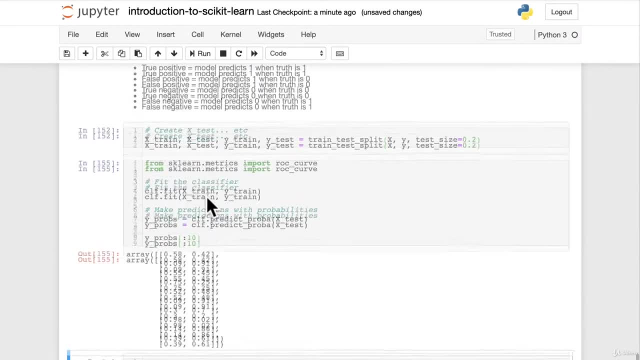 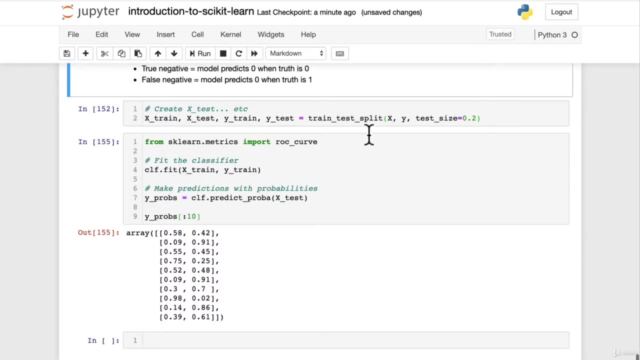 Okay, beautiful. And so because ROC curve only is a comparison of a model's true positive rate versus a false positive rate, we only want probabilities that the model has predicted for the positive class. So if you imagine here our model's trying to predict 0 or 1.. 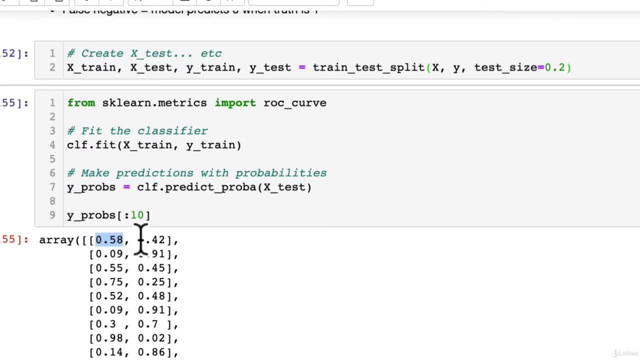 This is the probability that the label is 0. And this is the probability that the label is 1.. And so on for all of these samples until it finishes up. So there's going to be however many are in the test set here. 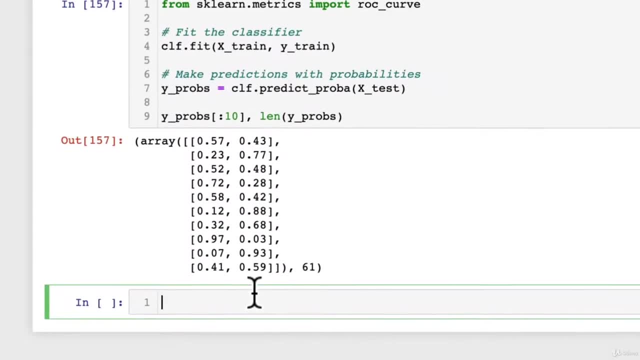 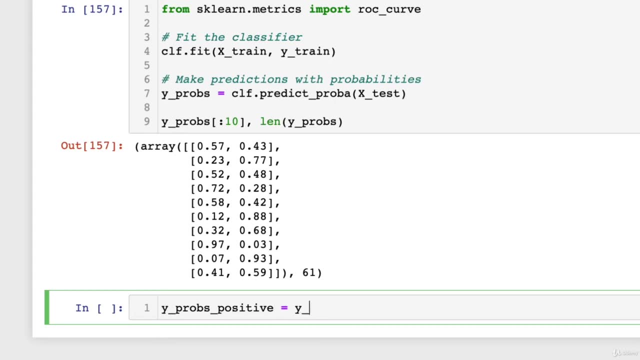 61.. So there's going to be 61 of these. So essentially, what we want is yprobs positive, So this is the probability that it's the positive. This is the positive class, aka 0 is the negative class and 1 is the positive class. 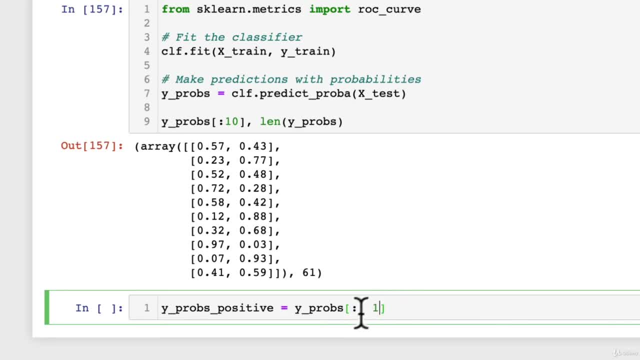 yprobs, we're going to use some slicing here, but only column 1 of every row. So that's, we can do that, Just so you can. you know what's going on. Positive, And we'll only look at the first 10 again. 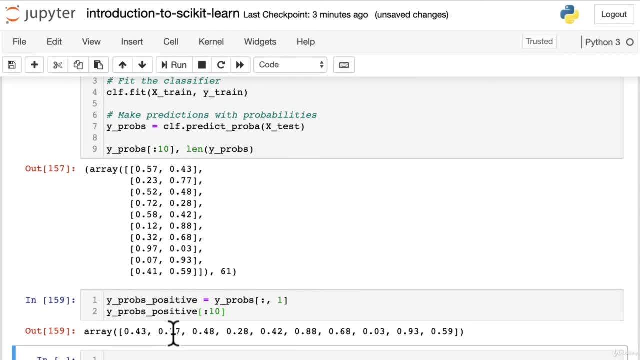 So does this make sense? We're getting 0.43.. Yep. 0.77.. Yep. 0.48.. So on, so on, so on. So this makes sense. We're getting 0.43.. Yep. 0.77.. Yep. 0.48.. So on, so on, so on. 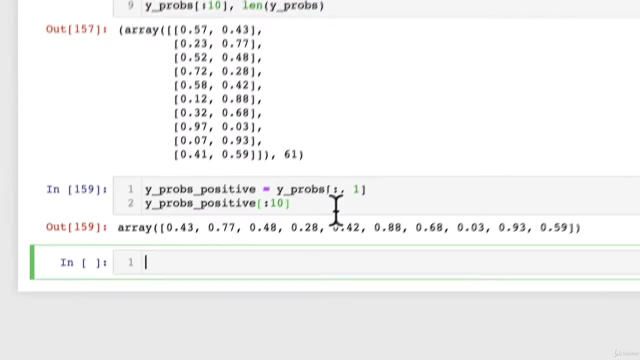 So this makes sense. We're getting 0.43.. Yep 0.77.. Yep 0.48.. So on, so on, so on For the entire list of yprobs. And now we can calculate FPR, TPR and THRESHOLDS. 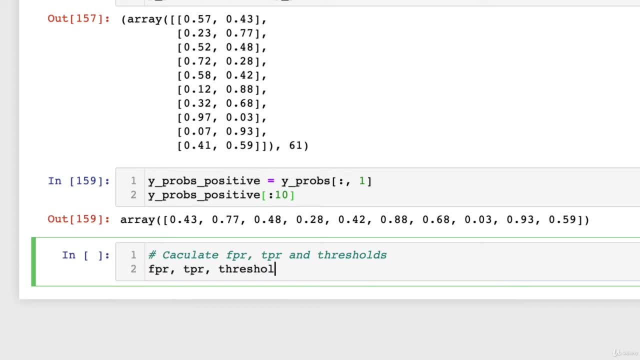 So we'll go? FPR equals TPR THRESHOLDS. Why do I know this? We'll see this in a second. Why do I know that this is going to be FPR, TPR THRESHOLDS? We've got ROCKCURVE. 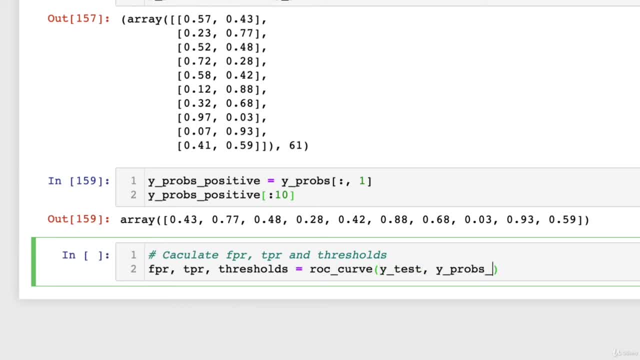 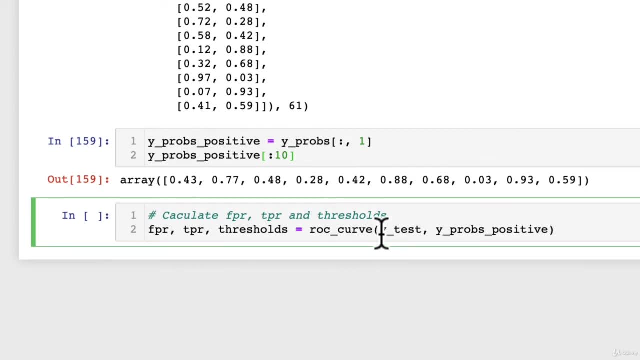 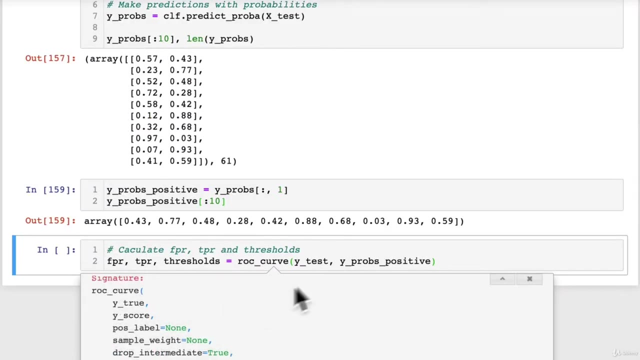 We're going to parse it yTEST and yprobsPositive. Now how would you figure out what rock curve returns in this case? Well, what I would do is I'd press Shift Tab and this is how I know. So we got rock curve. it takes Y true. 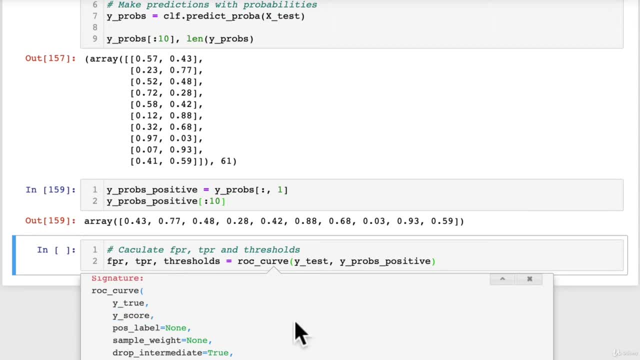 so that's our test labels. It takes Y score, so that's our Y probes: positive. And if we come down here compute the receiver operating characteristic rock, Yep, beautiful. Now parameters: Y, true Y score. target scores can be either probability estimates of the positive class. 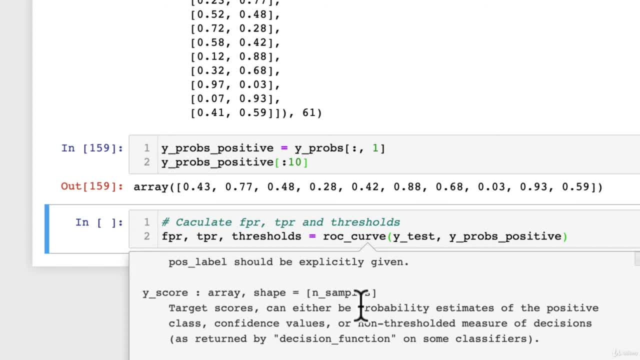 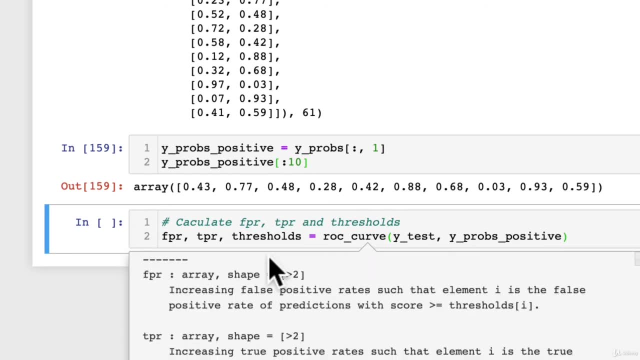 confidence values or non-threshold measures of the decision. So that's the probability estimates of the positive class. That's where we got this slice from right, And then if we come down here it's gonna tell us what it returns. FPR: increasing false positive rates. 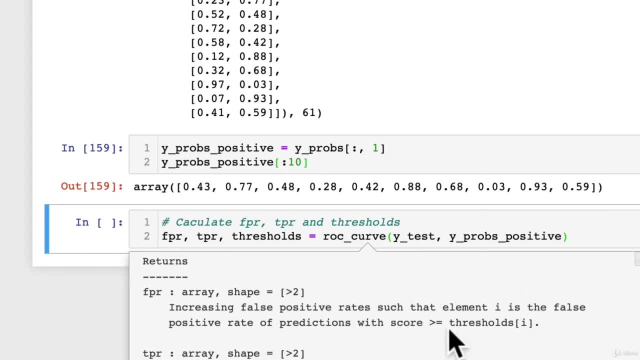 such that element. I is a false positive rate of predictions with score above thresholds TPR. so that's a true positive rate and thresholds. So that's how we can figure out what a function returns. And again, that's just viewing the doc string in a Jupyter notebook.